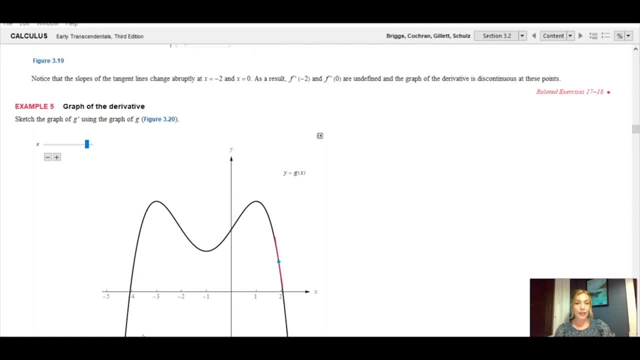 So what you're seeing on screen is from the calculus e-text, completely composed in Mathematica by Briggs, Cochran, Gillette and Schultz, And this is a replacement for the traditional paper book, And students come here to learn the concepts and then they would go to MyLabMath to work. 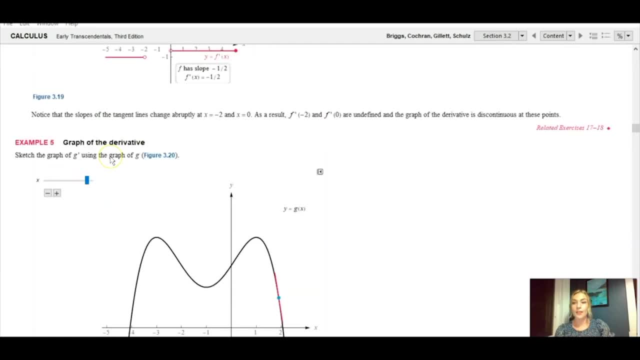 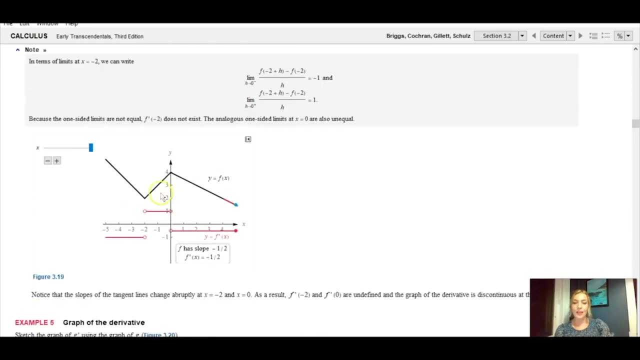 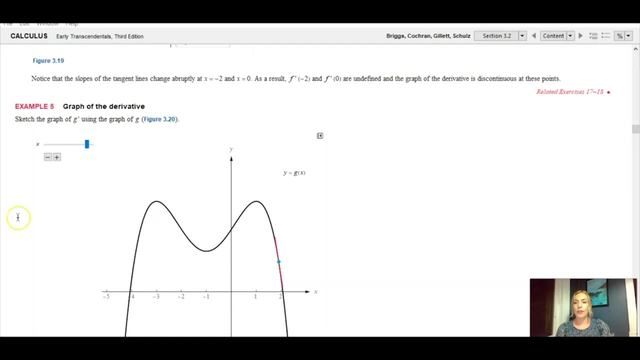 on homework assessment. This is chapter three on derivatives. So, as they're reading, the narrative text interspersed with practice. there are hundreds of these interactive figures woven throughout the narrative And for this example, we have a graph of the derivative and we've got some really lovely. 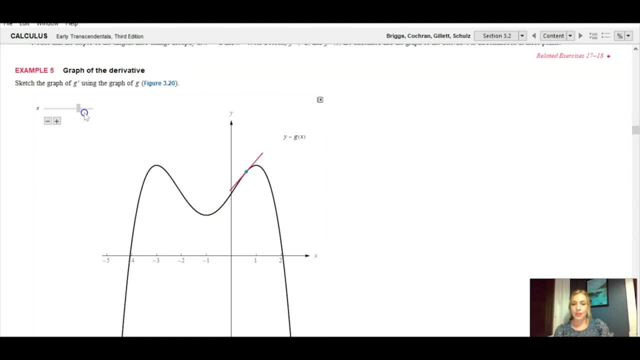 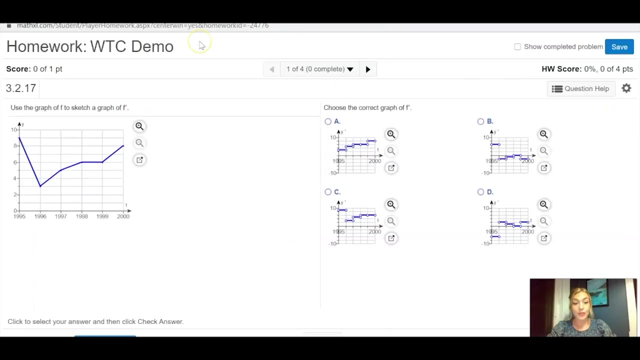 tangent lines illustrating the concept to students And, as I say, there are hundreds of these baked throughout the narrative text and, if you see, It suggests related exercises 17 to 18.. So if we hop over to the MyLab, we see what that question looks like rendered in the MyLab. 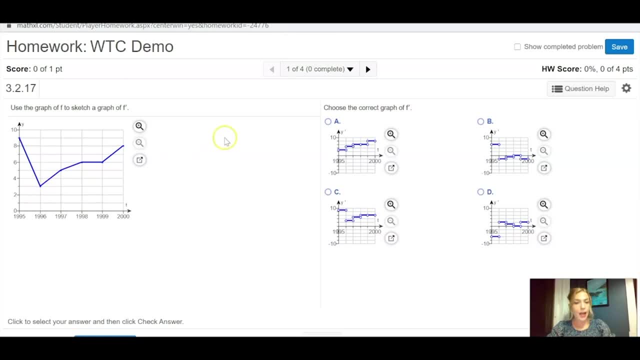 currently We have a static image and a multiple choice selection. for students, This is just not nearly as interactive as the experience they were just having in the e-text and doesn't encourage conceptual deep understanding of the concept. So let's take a look at what this question could look like using SILVA. 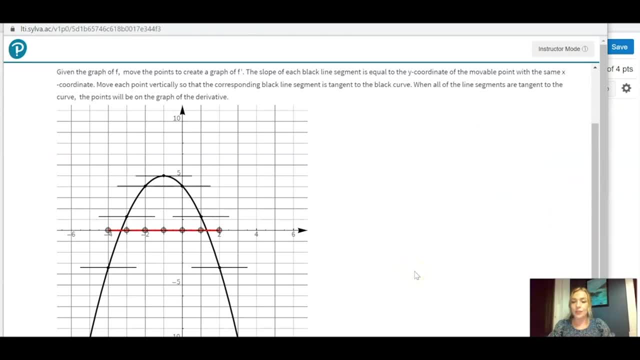 Here We have the same concept illustrated, only now students are interactively asked to graph F prime by moving these locator points. These types of questions, compared to what we just saw in the MyLab with the multiple choice, really drive home the concept of the tangent line and slope to students more than 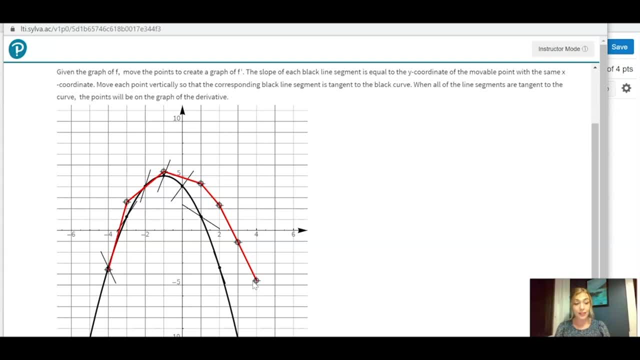 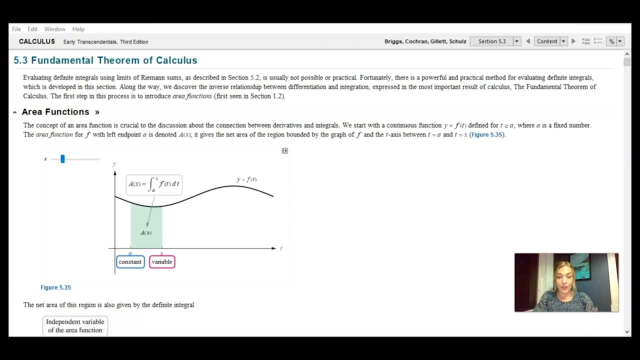 a multiple choice question ever could. So Let's look at another example. Here we are back in the Mathematica e-text, and this time we're in chapter five, learning about area functions. So once again, students are presented with narrative and the opportunity to see the concepts. 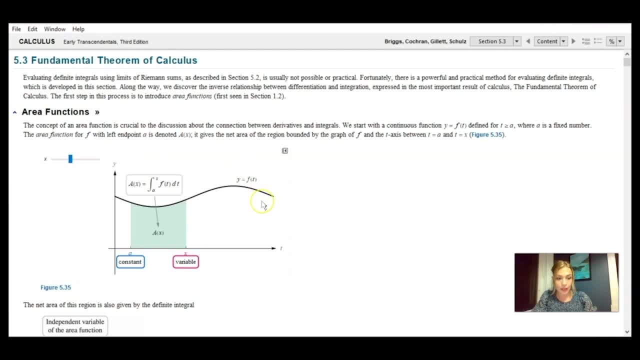 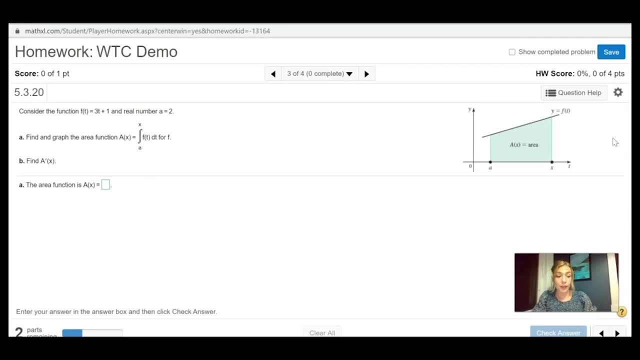 in action, using these interactive figures to essentially learn by doing Back in the MyLab. this is an example, a representative example, of the types of exercises that would be available for this concept. So we have a static figure Where students are asked to find and graph the area function which they would need to. 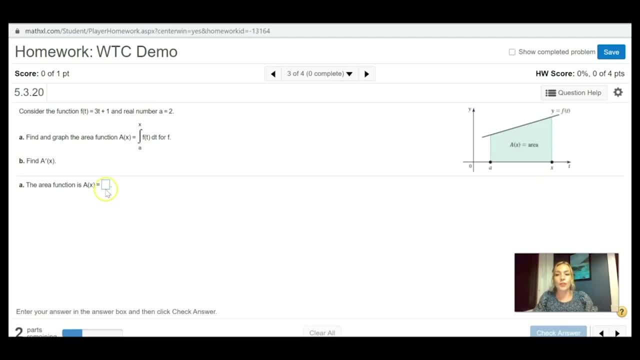 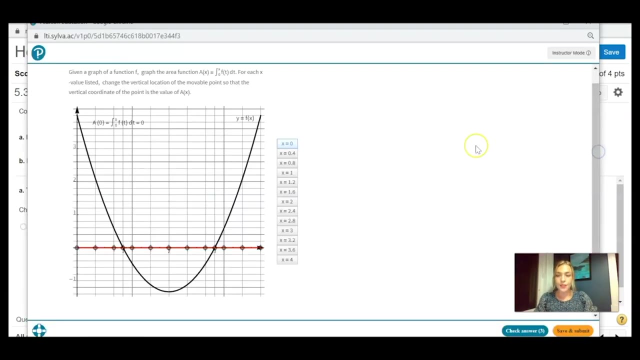 do on their own piece of paper and enter a free response here, followed by a multiple choice piece where they're matching. Now let's take a look at what this looks like as a SILVA exercise. Here, students are given the chance to interact and create the graph by moving these locator. 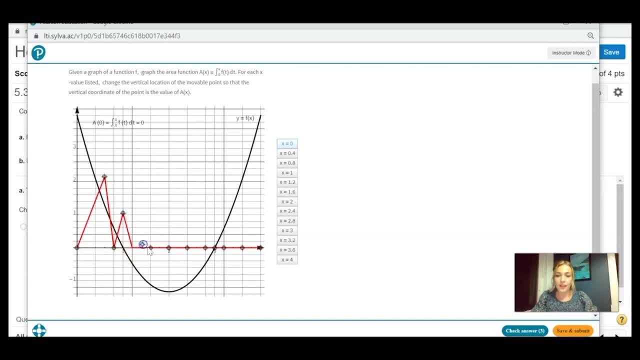 points. once again, They're able to see an immediate impact of their actions on the graph, They're invited to play around with it and are, all in all, more engaged and hopefully obtaining some of that elusive conceptual understanding that is a consistent request from instructors. 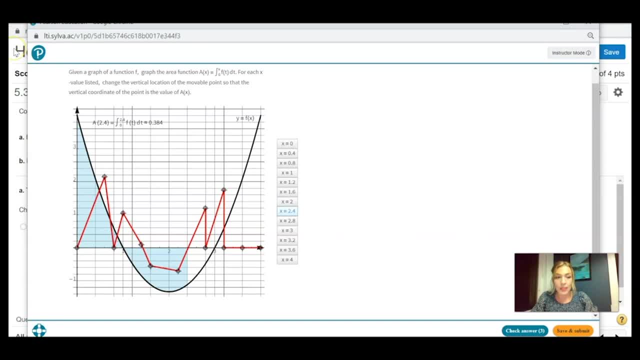 You'll notice that this is placed into a Pearson UI, So this exercise would sit along others in a student's homework. They're able to check their answer, receive immediate feedback and once they're satisfied with their answer, they would save and submit. 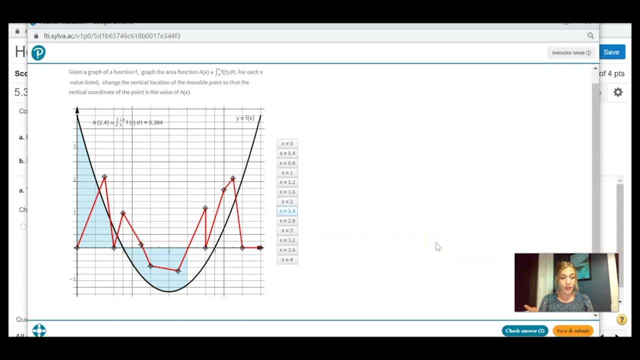 This would be scored alongside all of those hundreds and thousands of exercises that we currently have in the MyLab. So you would, as an instructor, you would be able to create an assignment, An assignment that did have some skill and drill exercises, perhaps a video assignment. 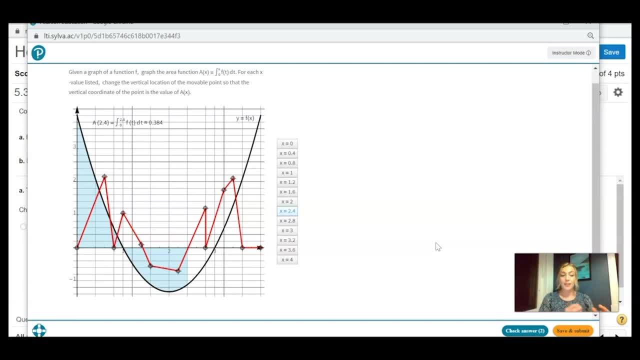 mixed in with some of these interactive style questions, some skill maintenance style questions, So you could devise an assignment that was more than just drilling the skills from a particular section. You would give students the opportunity to watch a little, do a little, learn a little. 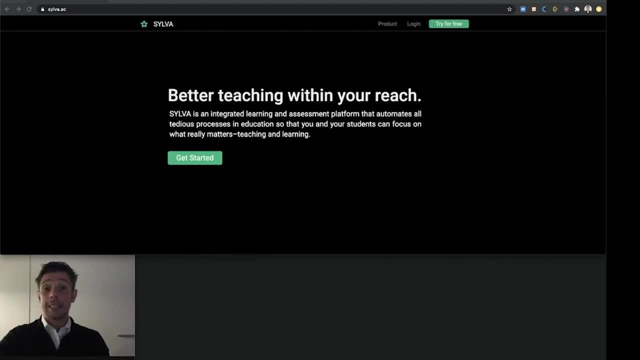 Thanks, Chelsea. We are really excited to connect with you. Thank you, We are happy to collaborate with Pearson to make math exercises more engaging. It's great to see what the Pearson authors already achieved with Silver, And today I want to show you a few more insights on how it works, how we set up questions and 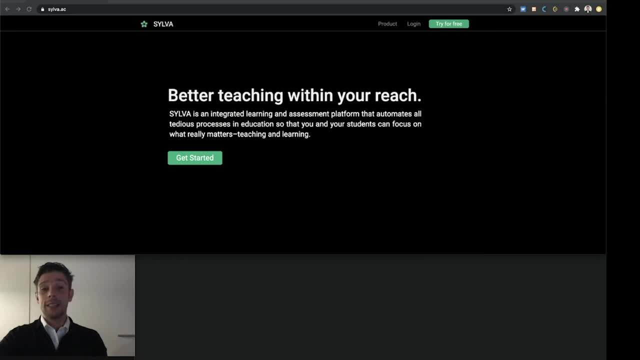 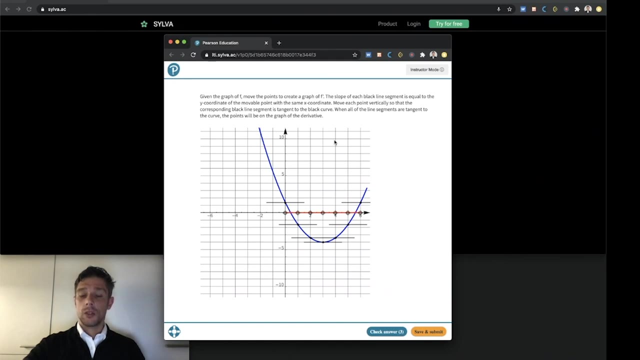 grading. Let me start by highlighting four main features Silver offers to authors. Number one is interactivity. Let's look at the example seen earlier Here. the authors took full advantage of all the powerful features Mathematica offers, such as creating dynamic interfaces in combination. 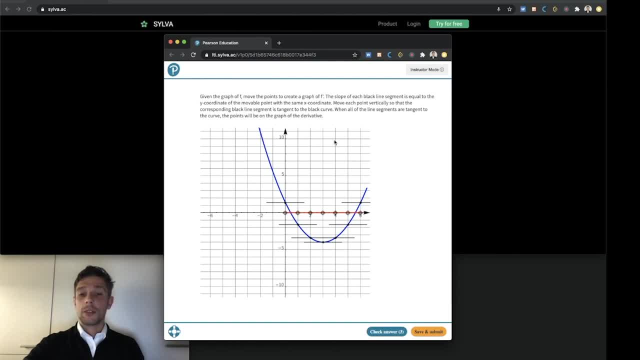 with graphs And with that they created a truly interactive experience for the students. As they moved the locators, the slope of the black lines would immediately adjust. This is interactivity. Now imagine a student would like to exercise a little more. 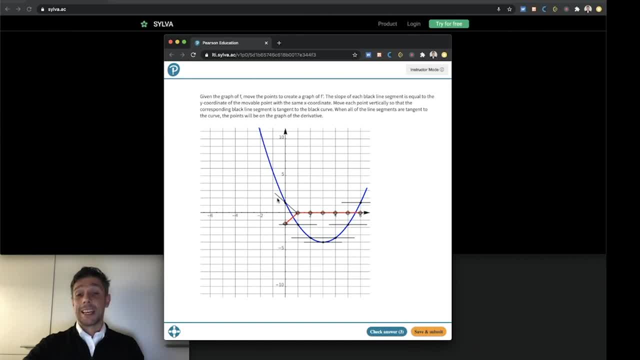 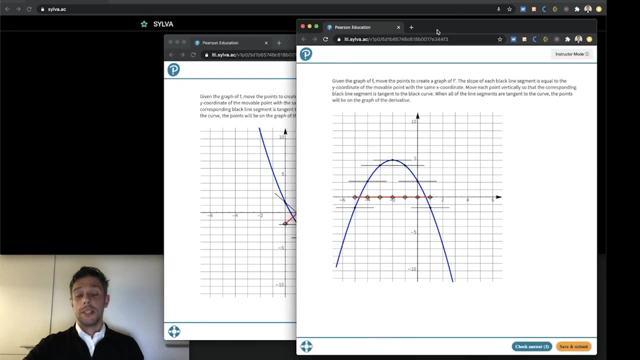 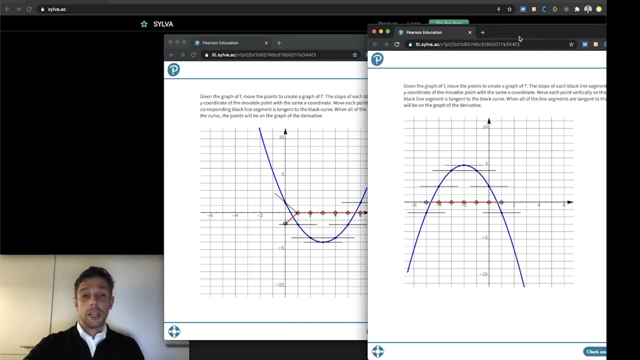 Then it would be really boring if they would always get the exact same question, And for that we offer parametrization and randomization, That is, creating different but similar versions of one and the same question. Here The task is the same, but the numbers change. 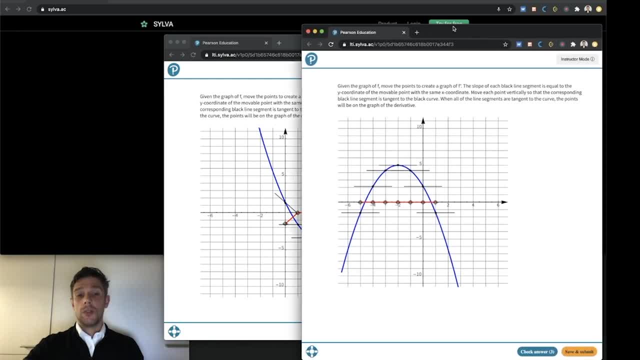 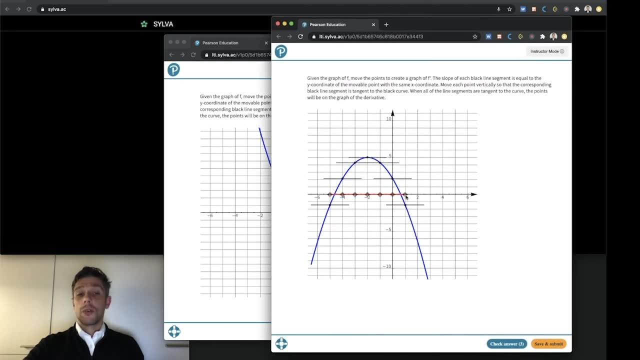 the graph is mirrored, and so on. This is parametrization and randomization. Number three is the autograding. Let's try to solve this question. As I move the locator, I see here now the black line is tangent and, as we know, the derivative. 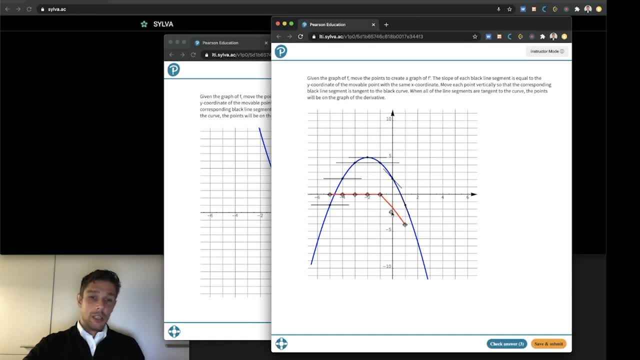 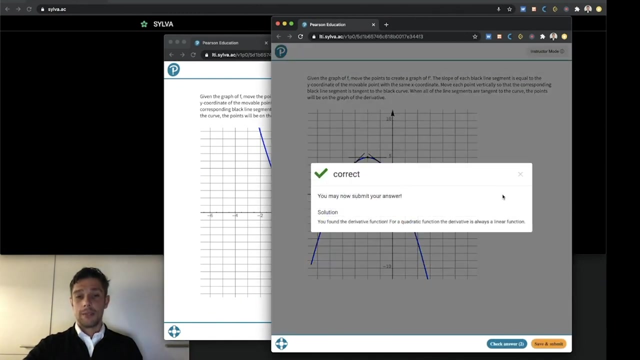 of a quadratic function is a linear function. So let me try to get this right. All right, Let's check our answer. And it's correct. We get an additional explanation. You found the derivative function for quadratic function. The derivative is always a linear function. 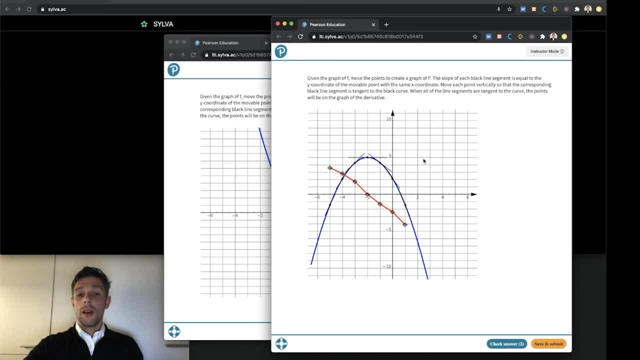 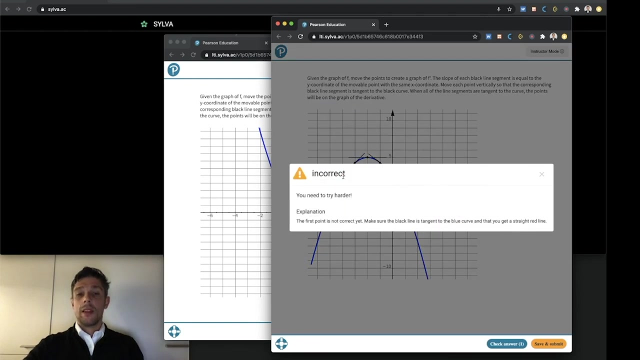 Now, this is autograding. What is really important for the learning experience are the cases where the student doesn't get it right. So imagine they would forgot to move the first locator. Let's try this Now. they get feedback that it's incorrect. 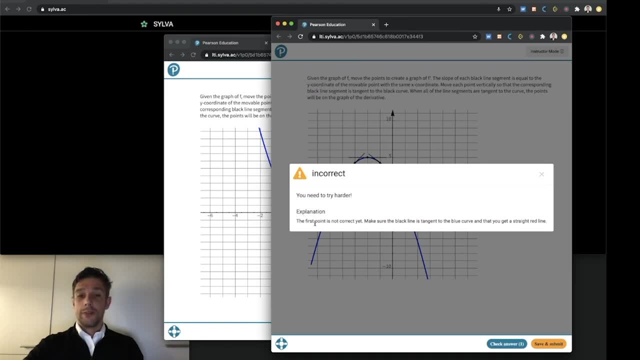 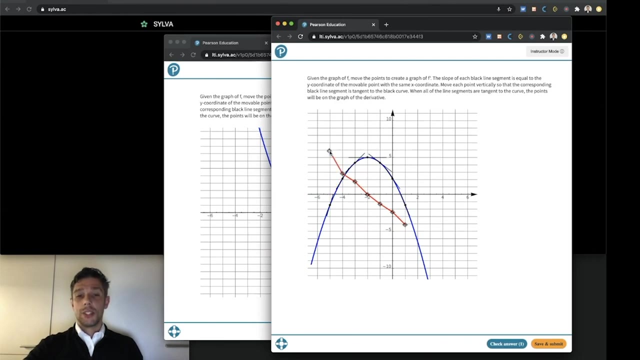 but with a tailored explanation. The first point is not correct yet. Make sure the black line is tangent to the blue curve and that you get a straight red line. Now let's do this, And now we get a feedback that it's incorrect. 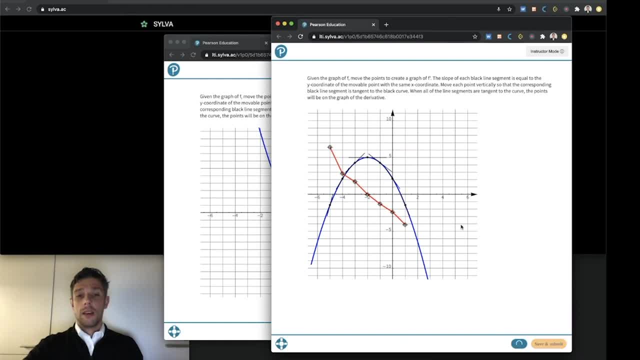 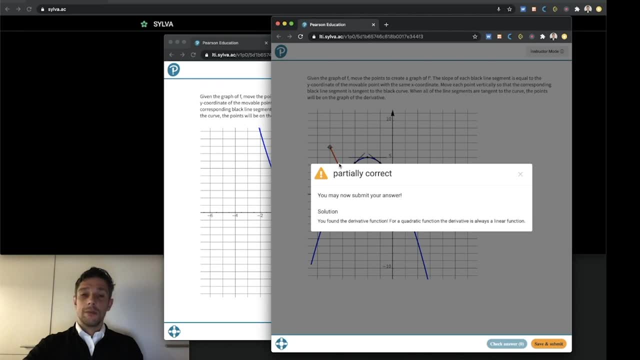 So what we're going to do is we're going to use this one, And we're going to use this one, We're going to use this one. And now we see third case. it's graded as partially correct, So it's almost right, but outside of the error tolerance. 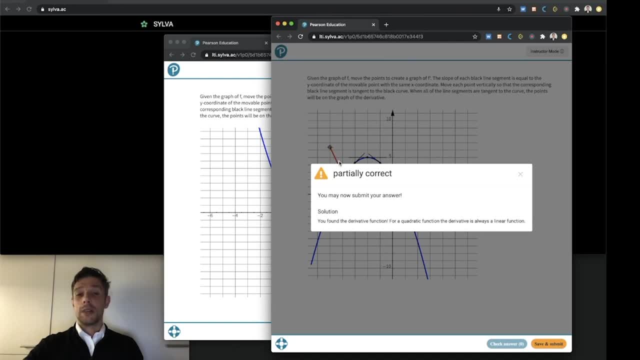 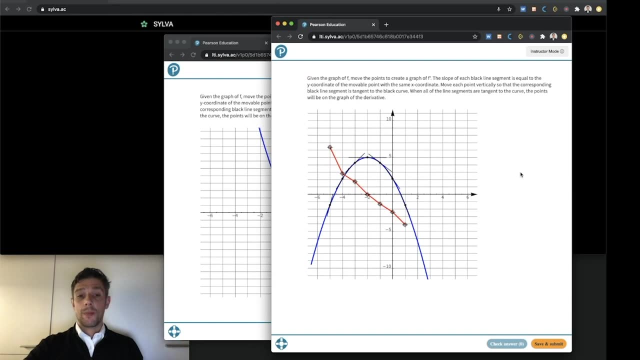 we defined And of course, that can be fully customized. That's number four, tailored feedback. And now you may wonder: how do we create such questions? At Silver, We want to equip all educators with some mathematical knowledge, with a tool that they can create such questions. 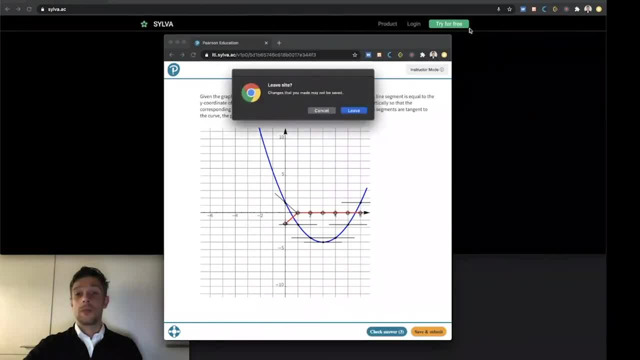 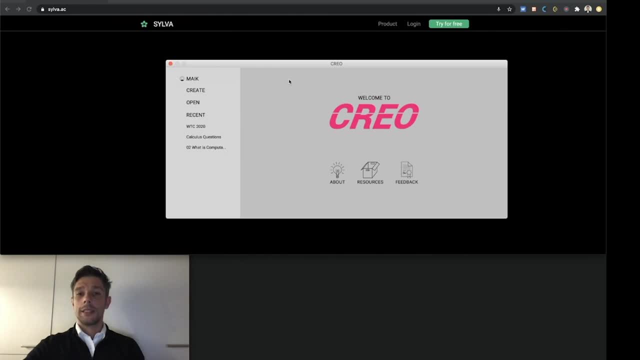 And for this purpose we created Creo. Creo is Silver's authoring tool. It's an add-on to Mathematica and once you install it it will be available through the palettes menu. It takes care of all notebooks. 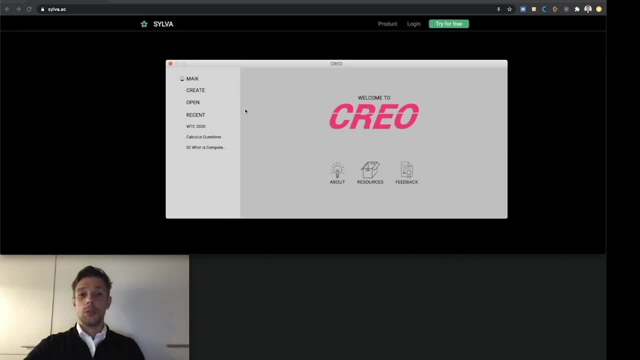 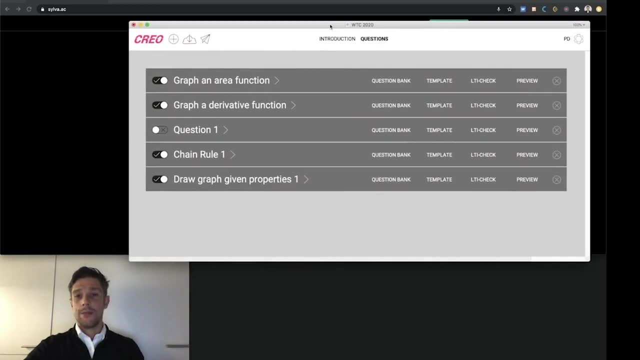 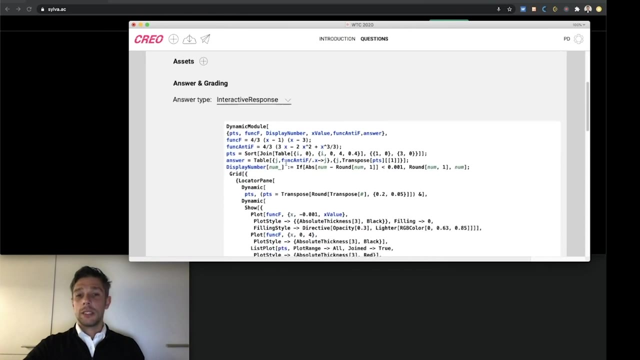 And files and questions and so on, so that you don't need to worry about it now, let's look at the notebook that created the question we have seen earlier. number one is graph, an area function. here you can see that once the dynamic content gets a little more deep, 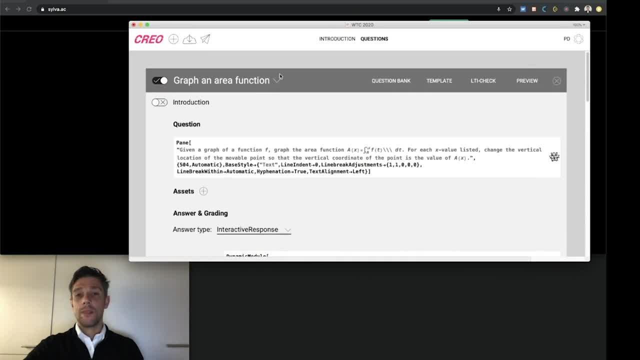 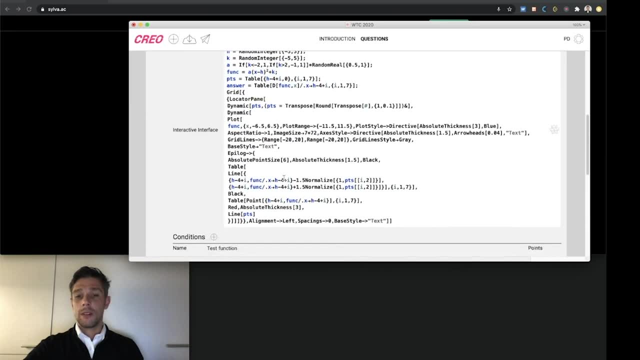 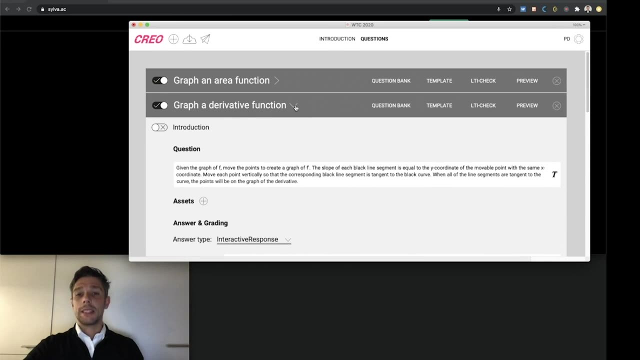 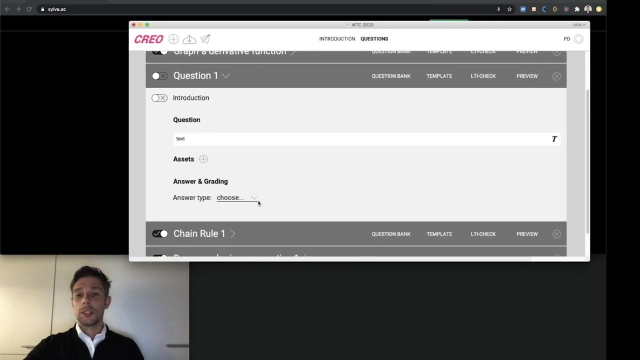 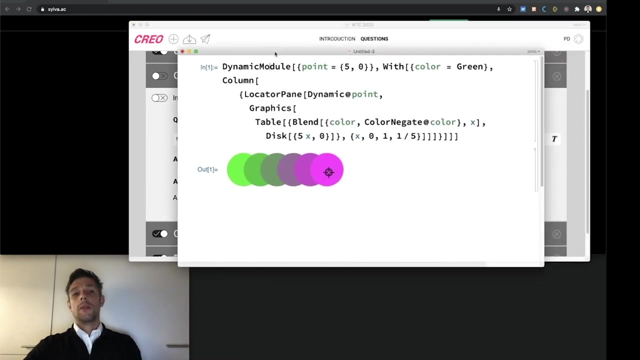 the code also will get a little longer. here is the second example. we have seen a little bit shorter, and here you also see the grading. but let's start with something easy, something from scratch. when you create a new question, it will just look like this, so assume you started with. 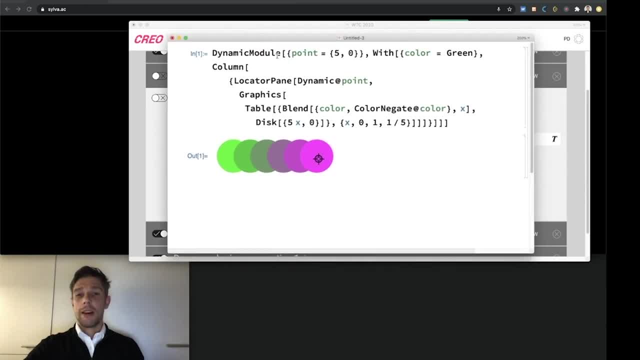 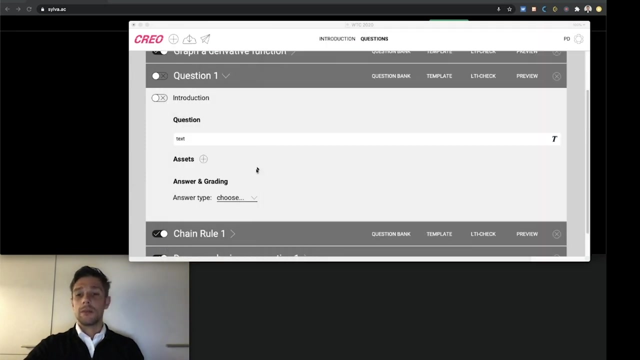 typing in the Mathematica notebook. here we have a dynamic module that includes a simple locator pane, some disk, and now we want to turn this into a question. how can we do that? we simply copy and paste the code into Creo. we want that it's an interactive question. 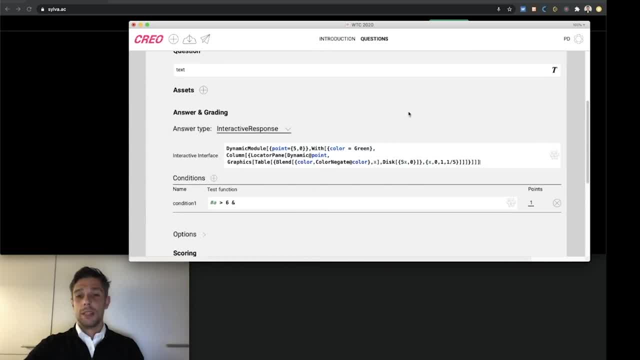 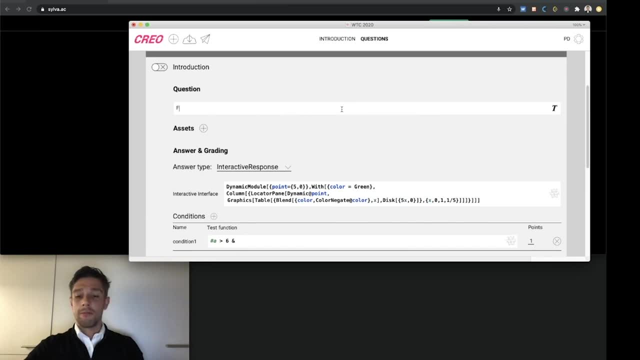 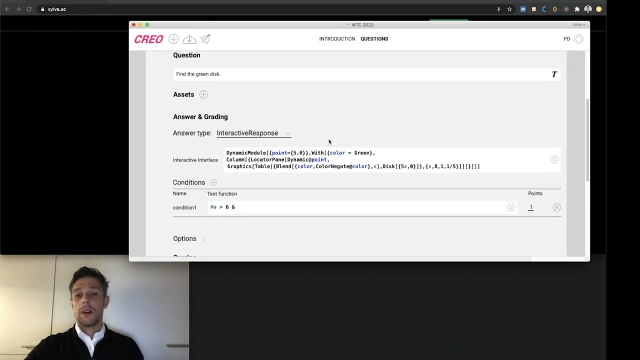 so copy and paste. that's it now. what kind of question could we ask about it? we could some say something like find the green disk okay, and now we need to look at the grading. here we defined a point and this is dynamic, so this will be our. 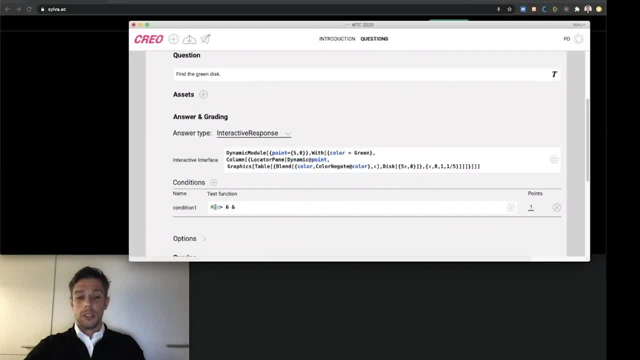 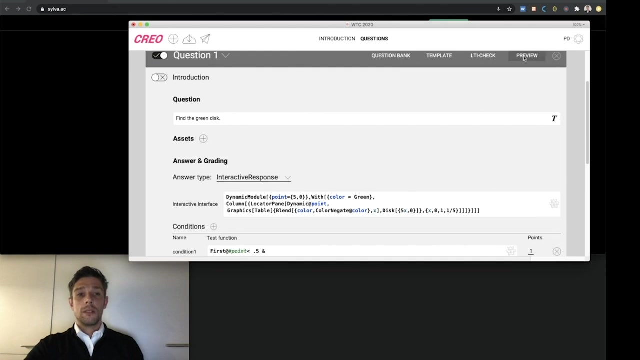 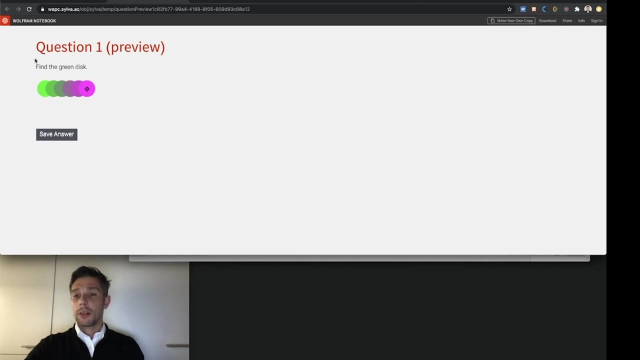 locator later. so what we can do is just say the point needs to be smaller than 0.5 and since we are interested in the x coordinate, put the first on that. all right now, let's preview this. so here we go. we have a question, find the green disk and we can move the locator and point it. 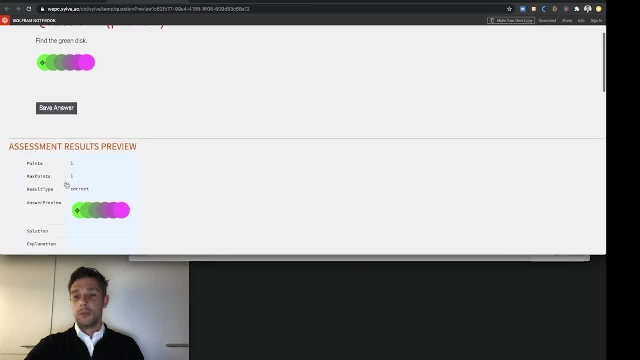 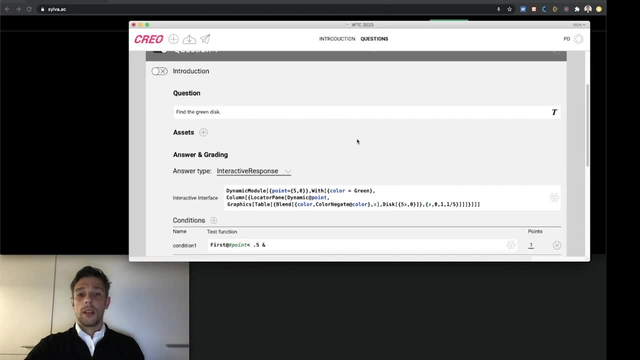 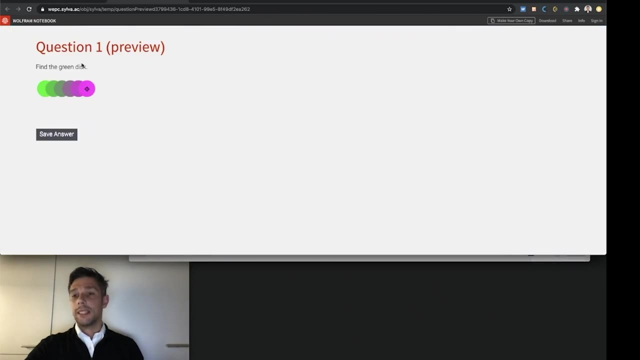 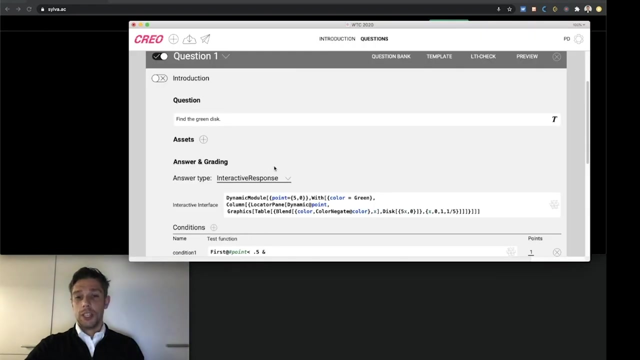 here to the green disk and we will get a correct. now, if we do this again, we get that. we will get the exact same question, and if we don't get it right, it will simply be incorrect. okay, now let's try to inject the parametrization here. in this case would be easy to just use. 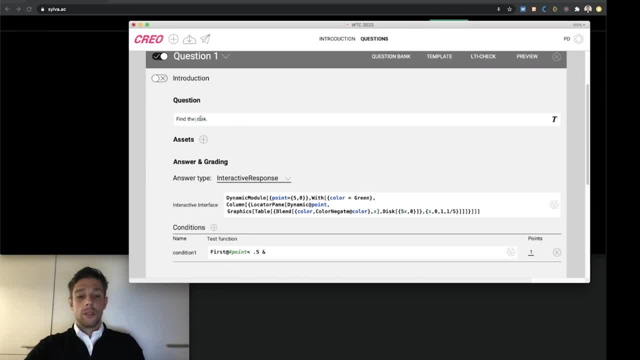 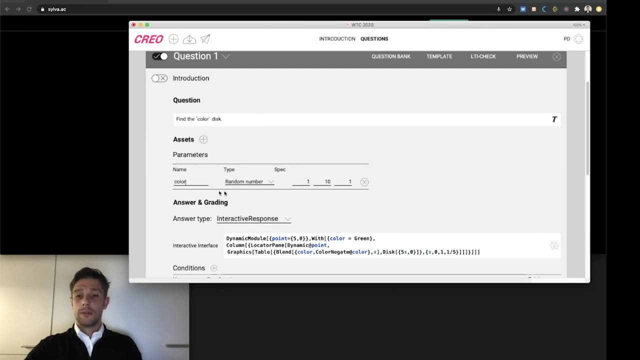 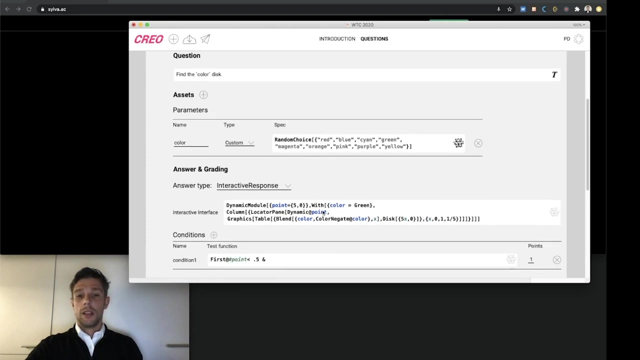 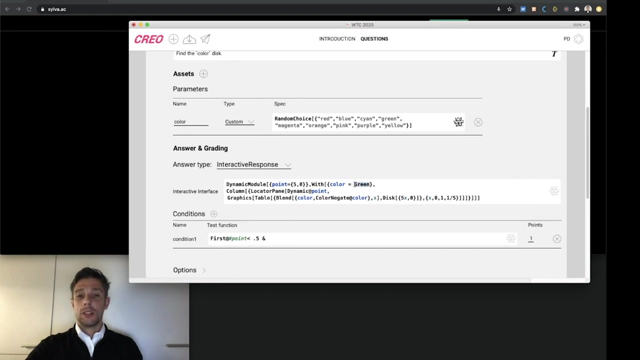 different colors. so let me replace the green with color and add a parameter. We call this parameter color and make it a custom list of colors: red, blue, green and so on. Now we want to inject this into our interactive interface. 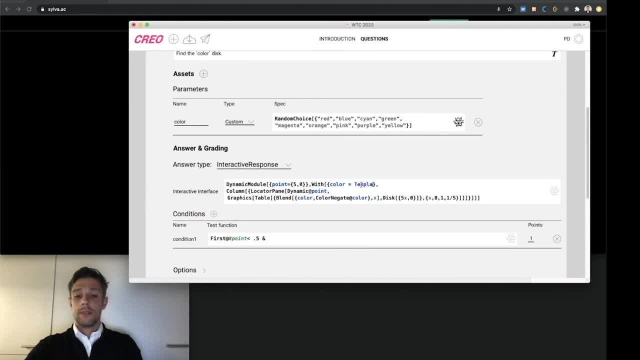 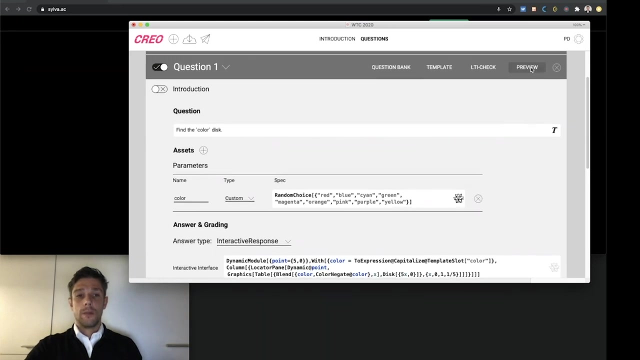 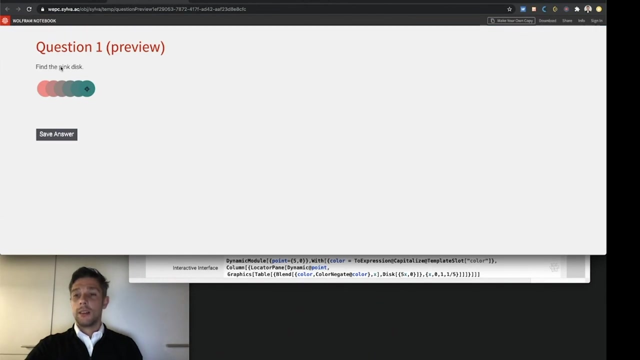 So we replace the green by template slot and then simply color. Now, in order that those colors get recognized, we add a capitalize And true expression in front. All right, Let's test this now. We see that we get immediately a different version. 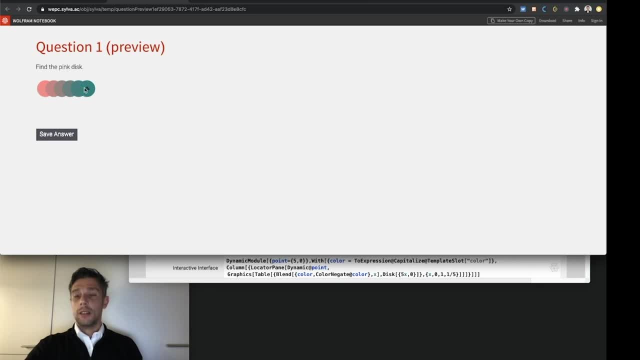 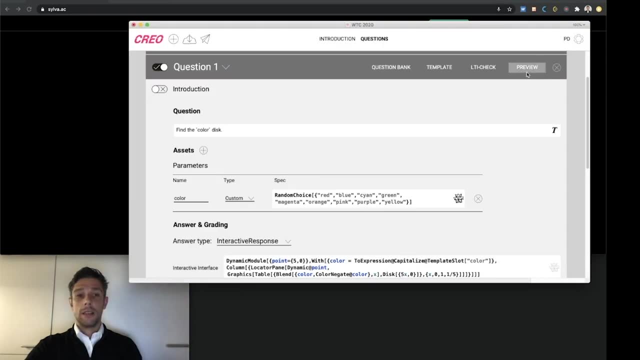 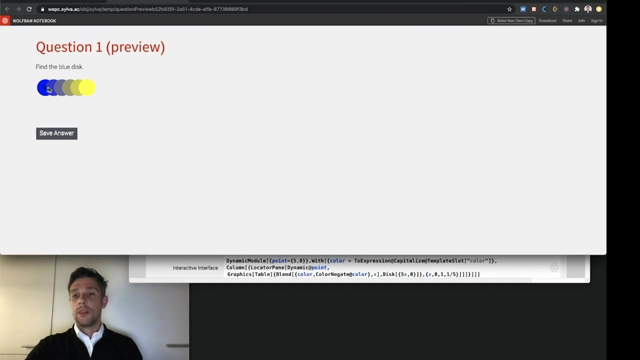 So now it picked pink one and created the nice color of this. So let's try another version And we get the blue one. So we injected the parametrization and randomization, but we still have on the kind of black white grading. 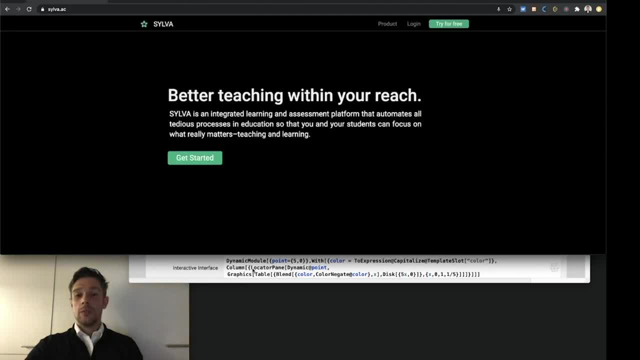 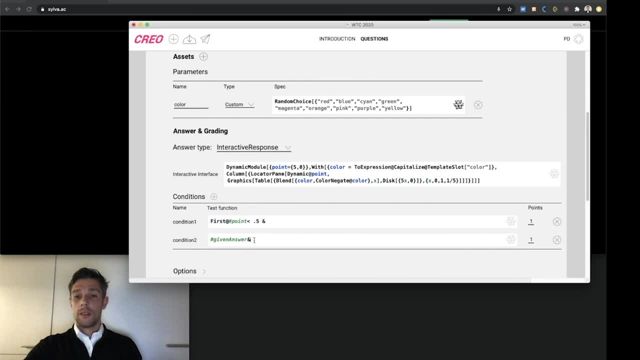 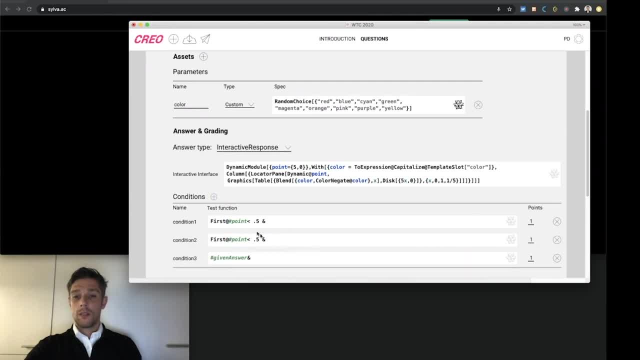 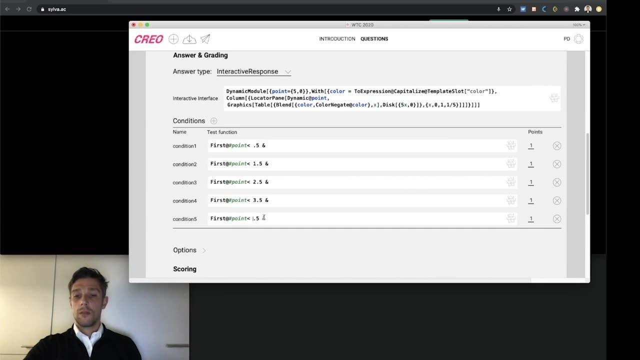 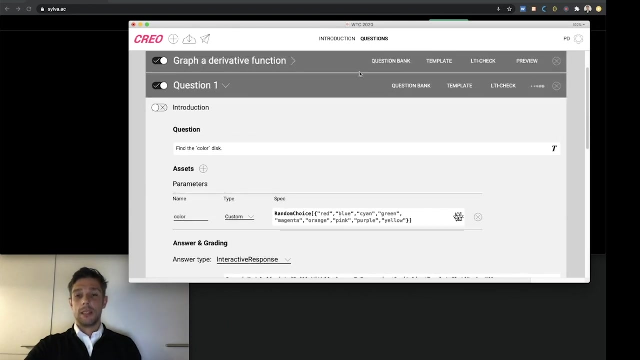 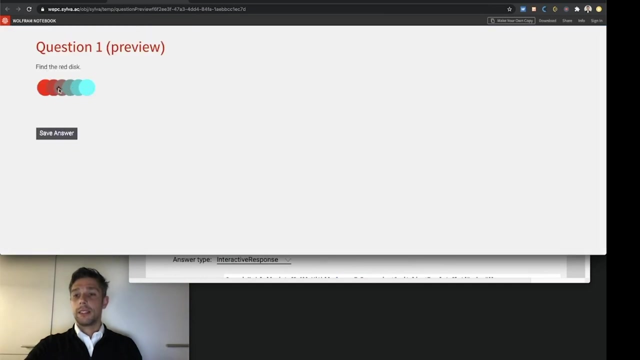 So let's add a few more conditions here. All right, Now we can test, all question again. We get a different version and let's see what we get when we get somewhere in the middle. Now this is considered partially correct and the grading works like this: 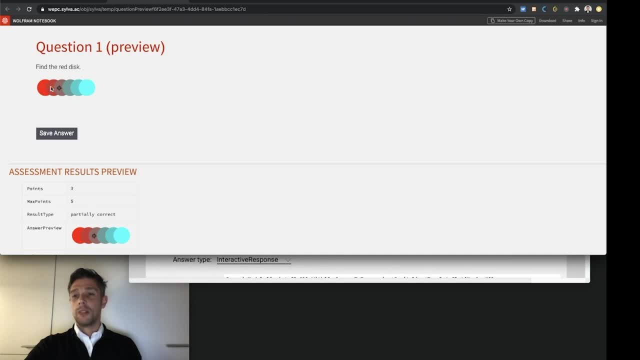 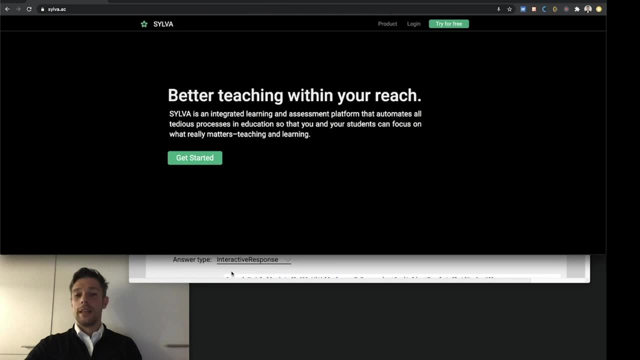 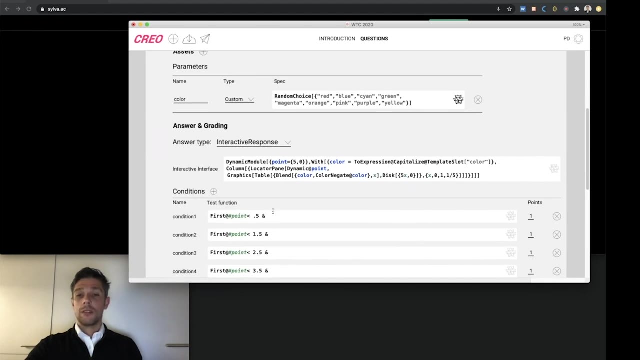 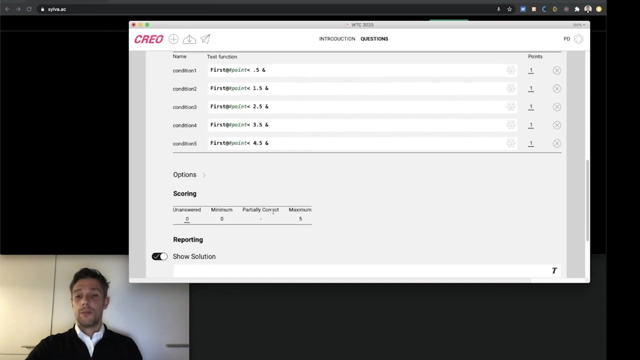 If you get the red one, you get four points and for each disk you're away you get one point deduction. Now we've set up a question with parametrization, with partial grading, but let's look at the feedback. now We have two fields. 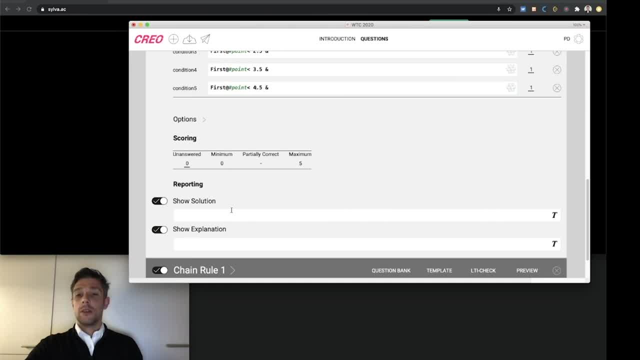 One is the solution, one is the explanation field. The solution is given when you either did not get it right after a couple of attempts or when you get it right at some attempt. In this case, we could just type something like well done, but that would be a very static. 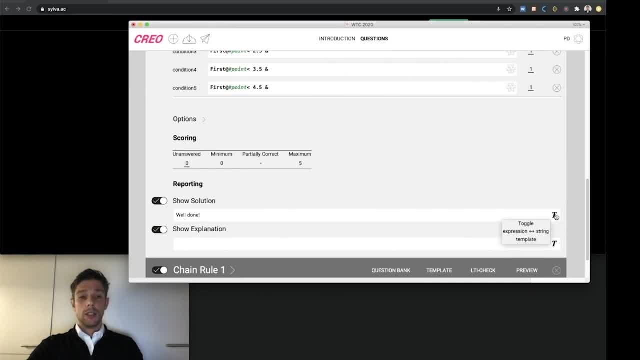 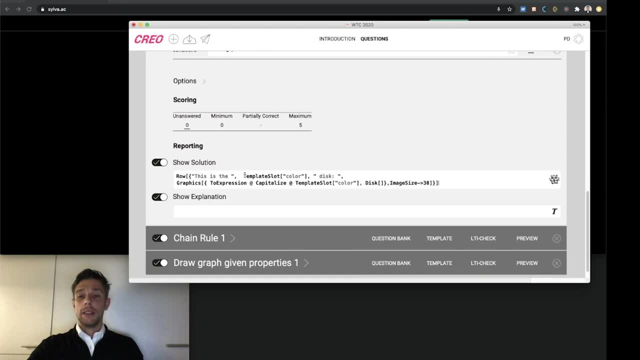 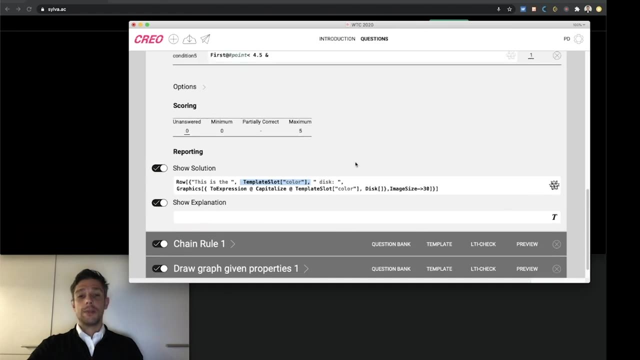 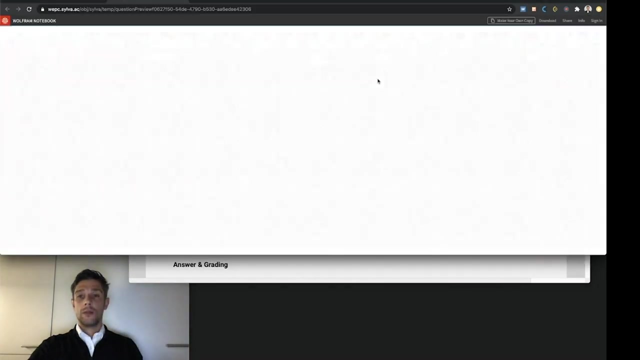 message. So instead we can toggle here and use an expression, So we could say this is, and then pick the right color disk and we could even show it. All right, let's test this. Now we can move here, get it correct and this is the right disk. 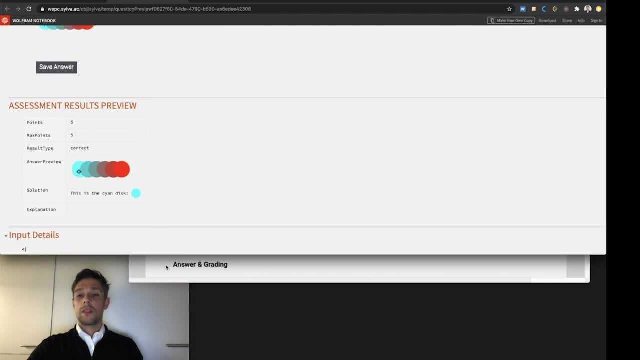 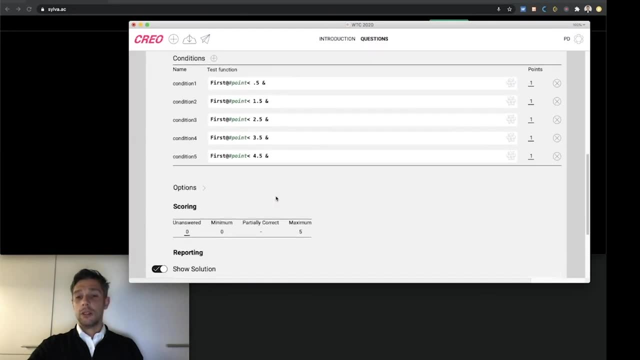 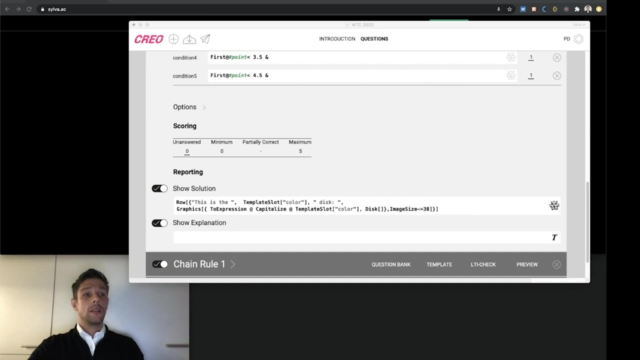 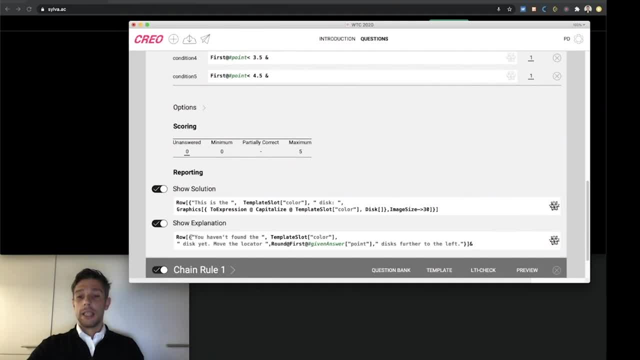 we can go even further. So here we can say: you haven't found the right disk yet, And then we can give tailored feedback by taking into account the answer they provided. So in this case we can extract from the given answer the point. 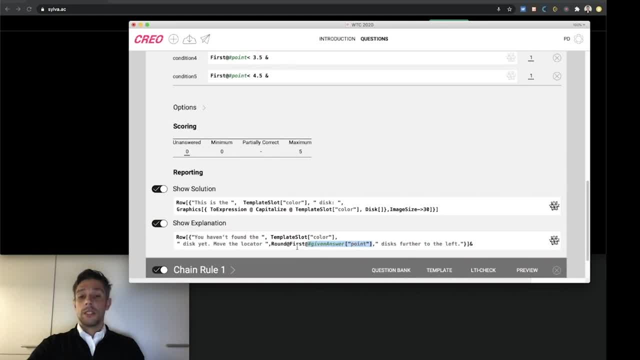 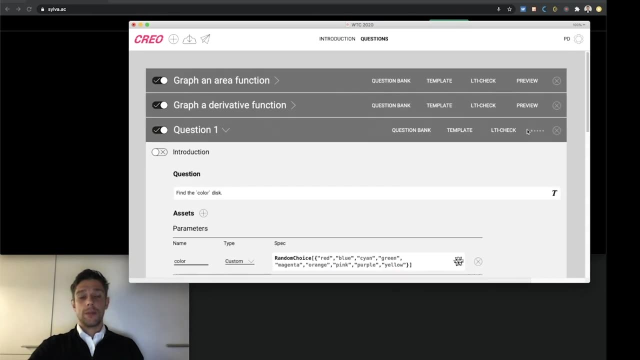 And, as we know, this is a coordinate, We take the first, the X value, again rounded, And this gives us the number of disks they have away from the actual solution. Okay, Okay, Okay, Let's try this, Okay. 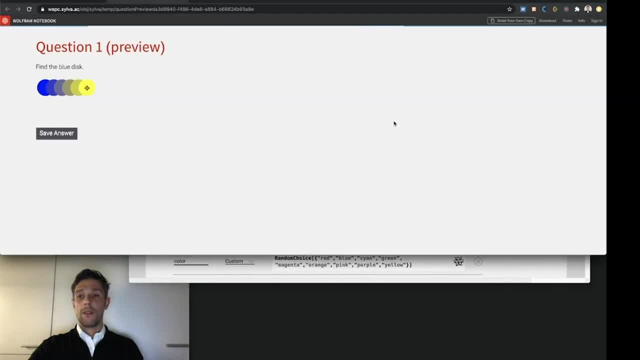 So I move it here in the middle, and this would be three disks away And we get. you haven't found the blue disk yet. Move the locator three disks further to the left, And this is how we can provide the right disk. 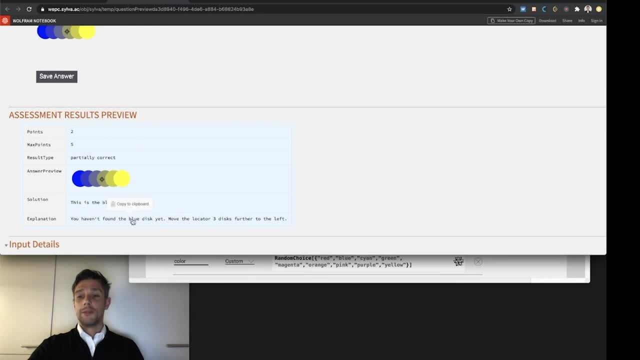 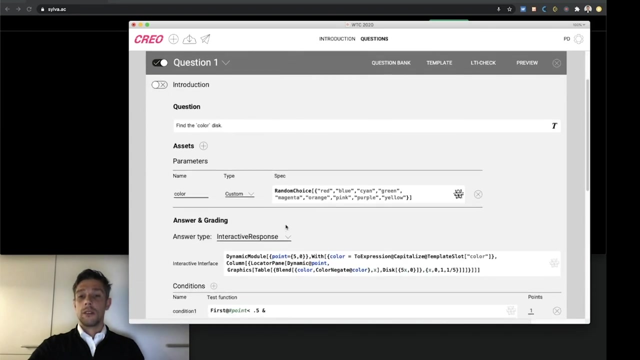 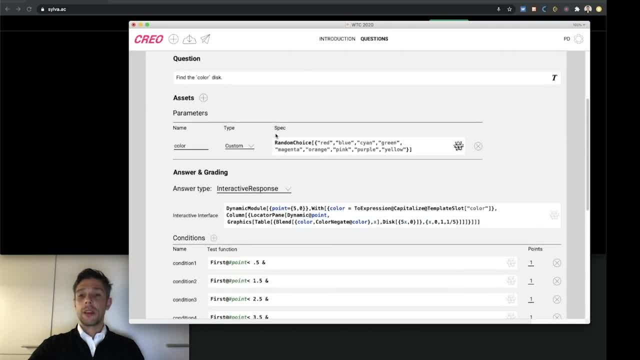 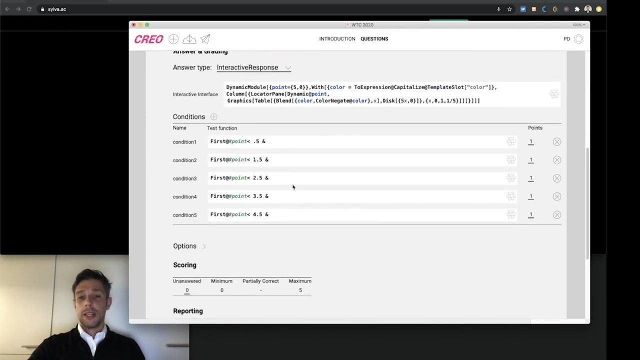 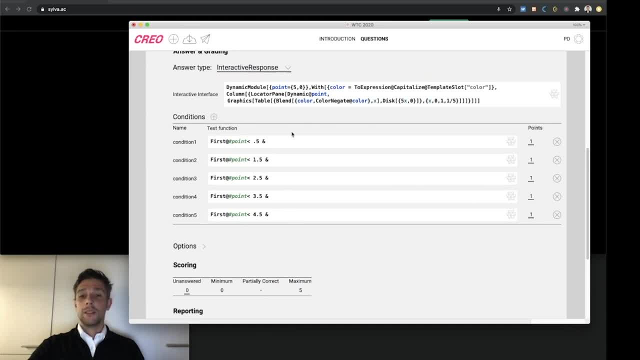 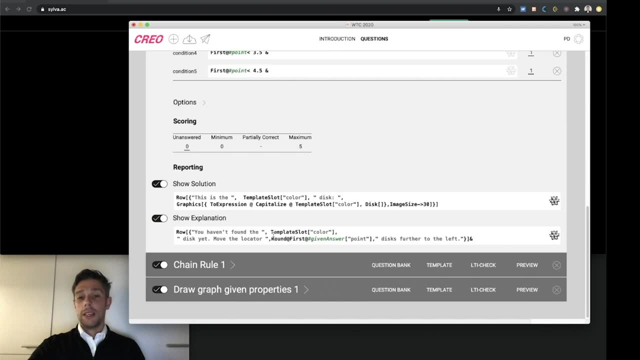 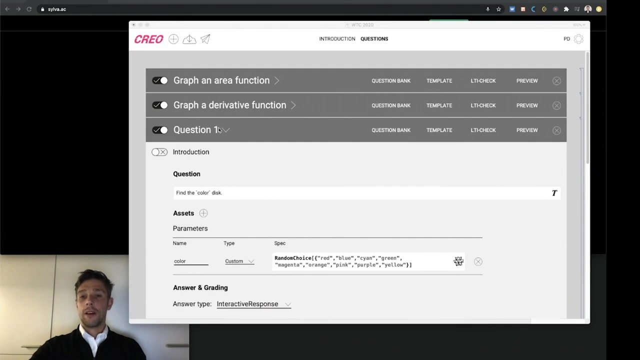 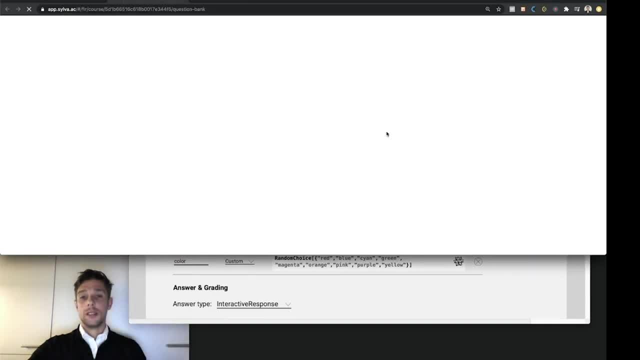 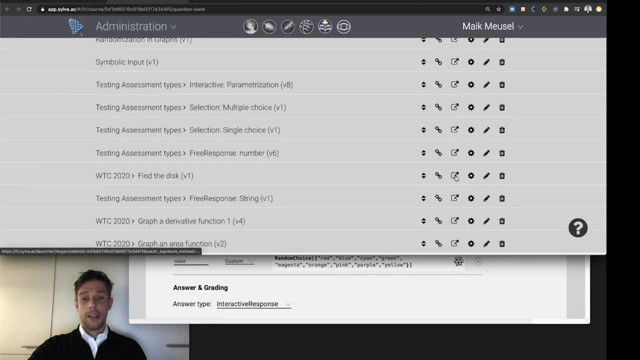 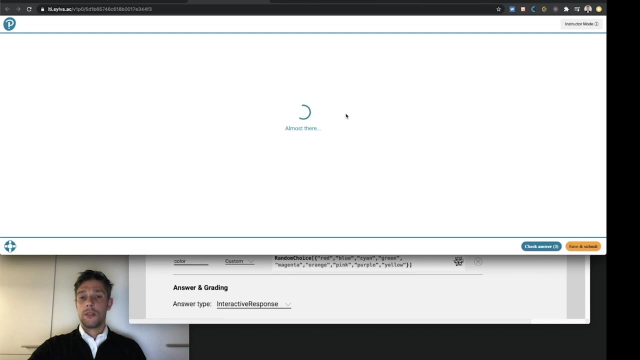 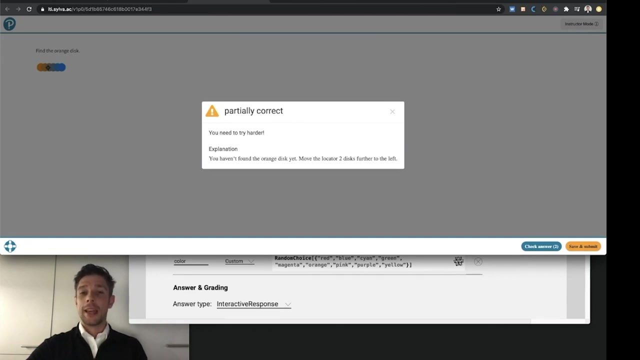 ask Creo to deploy, which is as easy as one click, And now what we get is a MyLabReady question. There's so many more things we can do with Creo, but let me hand over to Chelsea again to share some feedbacks from the authors with you. 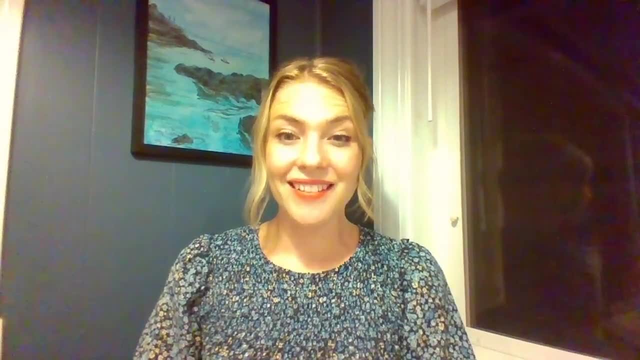 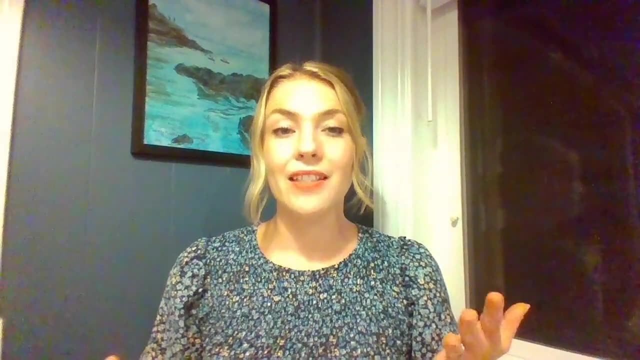 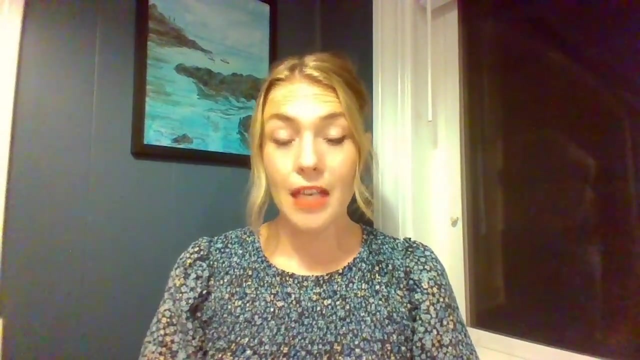 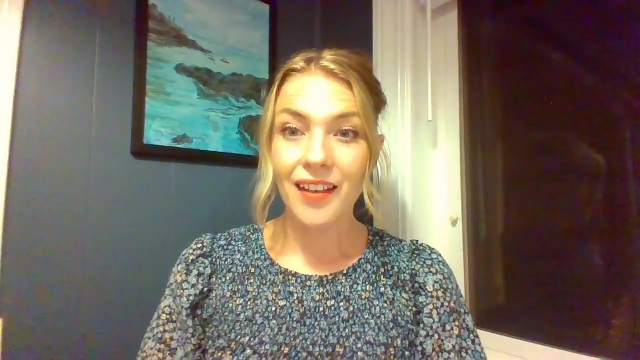 Pearson authors. Those are really excited by the possibilities. Eric Schultz, the co-author of the Calculus eText we viewed earlier, emailed me late one evening to say that he had written the Mathematica code which recognizes multiple parametrization forms for tangent lines to curves, with free form input. to boot multiple exclamation points. 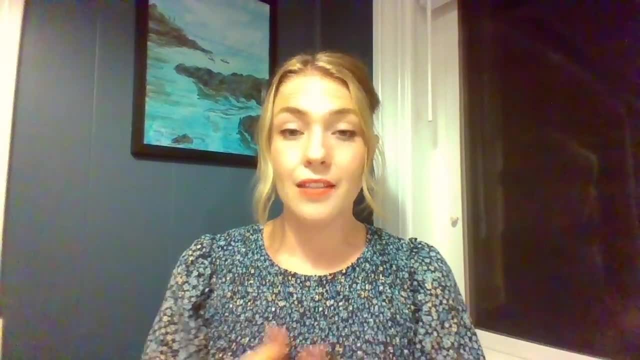 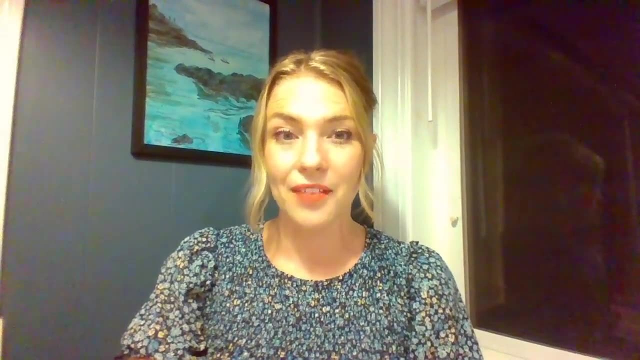 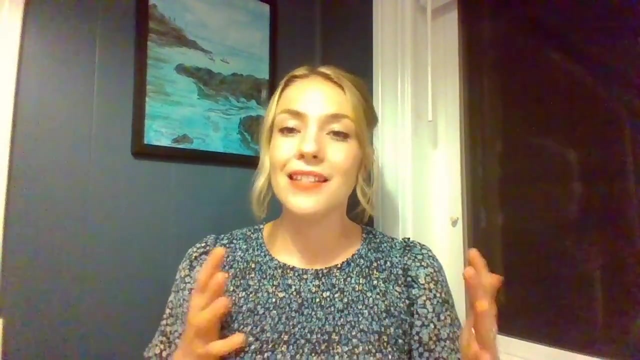 Our current MyLab exercises will typically ask for the standard parametrization form for the tangent line, So this represented a breakthrough for him on that particular question. A few days later, another note from Eric came in. Exercises in the textbook will often ask questions that we cannot exactly replicate in the MyLab. 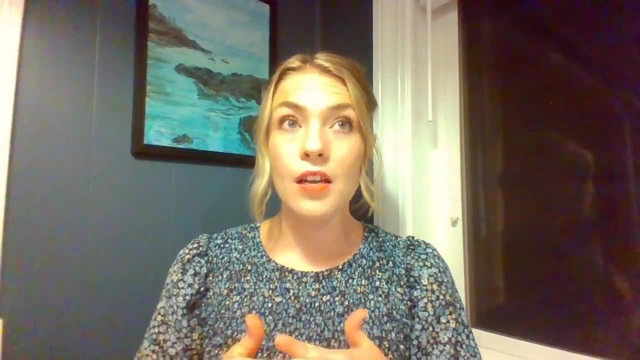 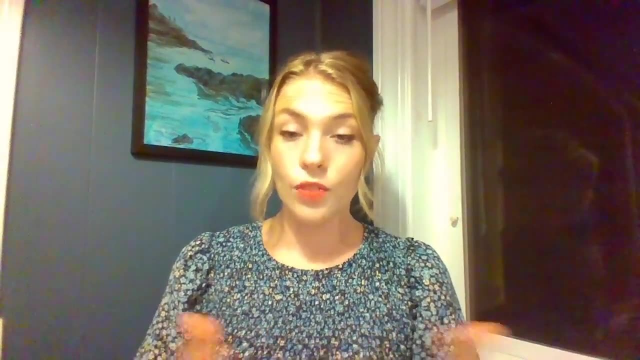 So consider an exercise that asks the student to sketch the graph of a function satisfying some properties Like Increasing, Decreasing, Increasing at a decreasing rate And now, etc. on this interval or that interval I like to call these. the answers may vary. 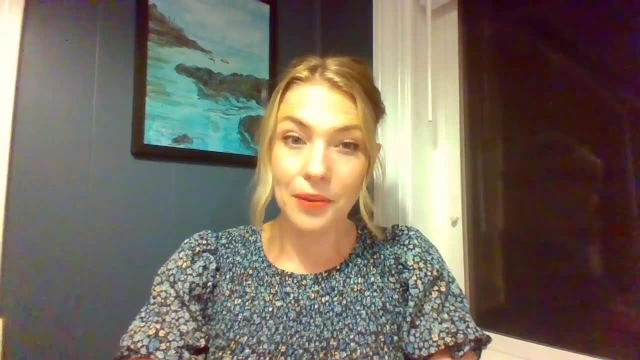 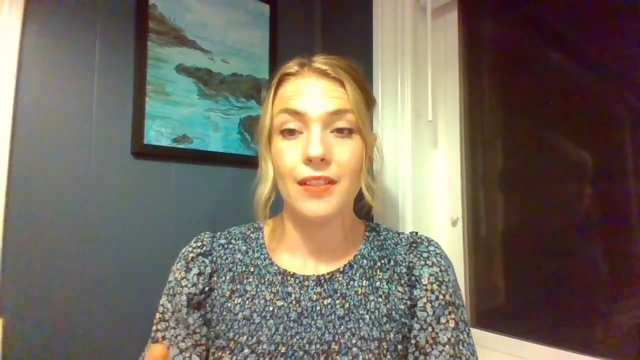 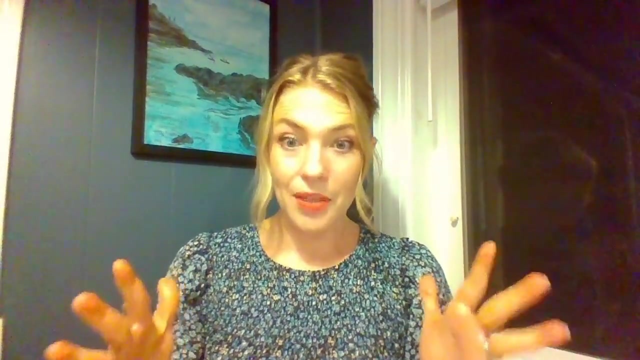 exercises, since that's what you would see in a solutions manual. So Eric has coded several new exercises in Creo that allow students to draw these functions that satisfy a set of properties and have their answers graded by Silva. So more exclamation point: These are exactly the kinds of exercises that instructors 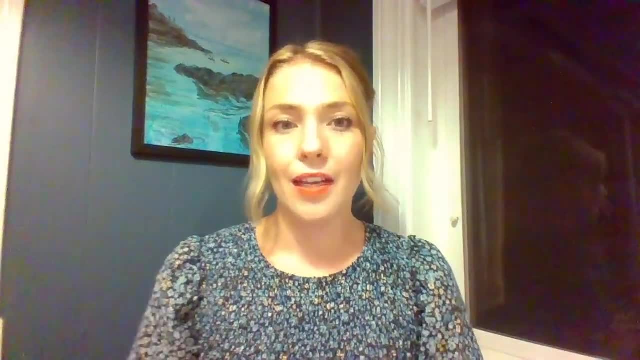 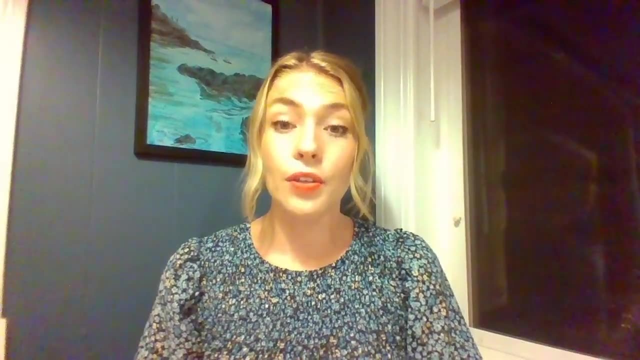 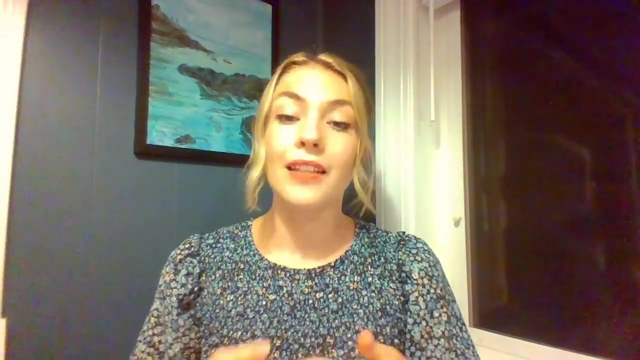 and authors slash. instructors would like to assign to students, but doing so on paper is not scalable and doing so in the my lab is not currently possible. So with these new tools it is and instructors will have yet another exercise type that they can assign to students. that drives that conceptual. 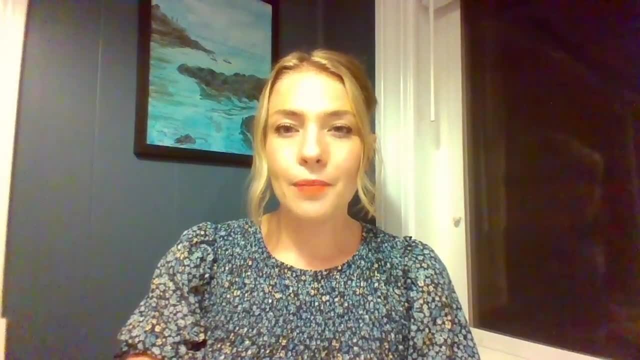 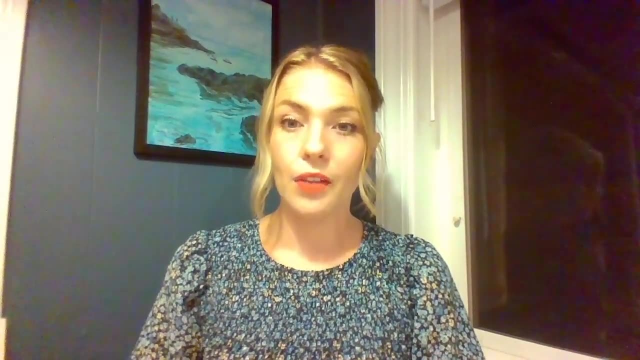 understanding. Another challenge we face in the my lab is interpreting student responses. So student responses are the ones that are most important to the students. Students use palettes in the my lab to enter expressions in a particular way and the system scores them very rigidly on what they entered. 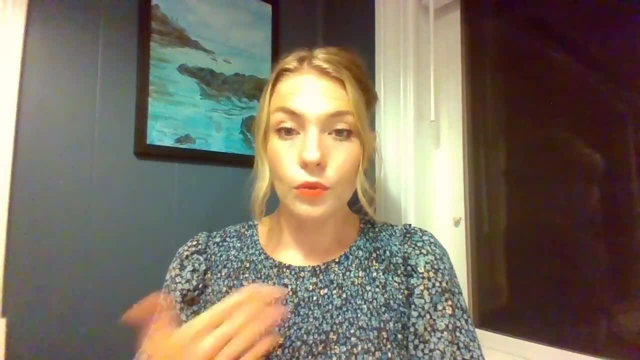 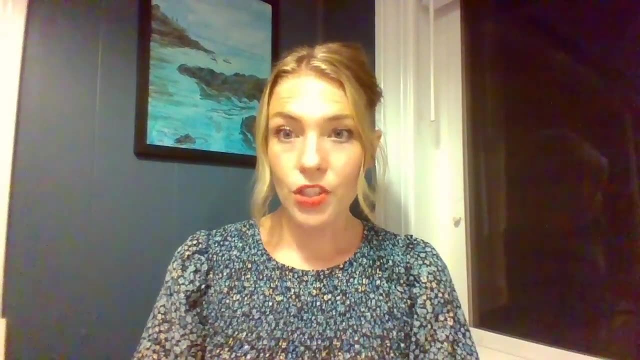 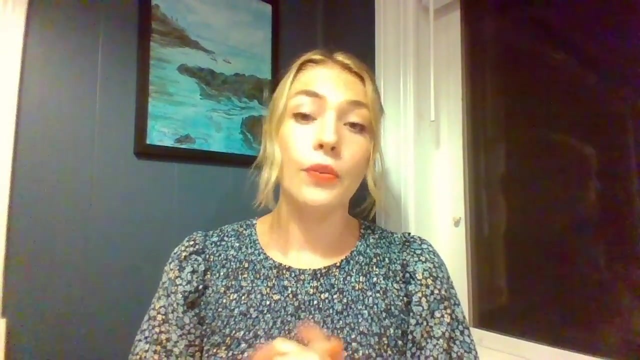 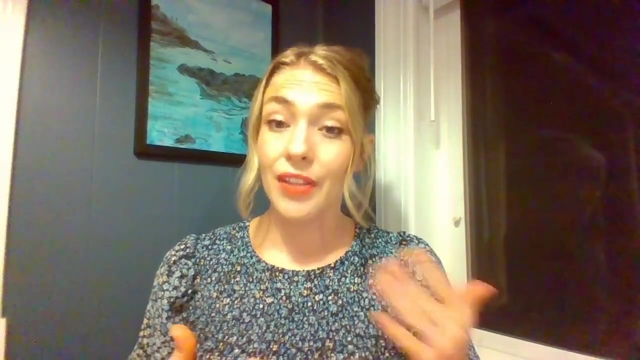 So by using Creo, it allows us to leverage the linguistic knowledge of WolframAlpha to interpret student input to exercises. So consider a randomly generated exercise where the answer is sine x, parentheses x. The following inputs in Silva would be accepted As correct, of course: sine parentheses x, sine with a capital, S parentheses x, sine.